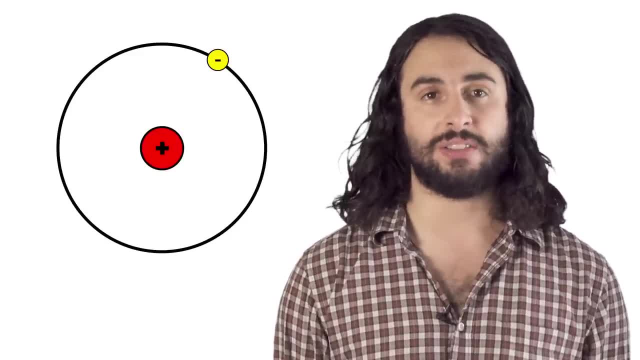 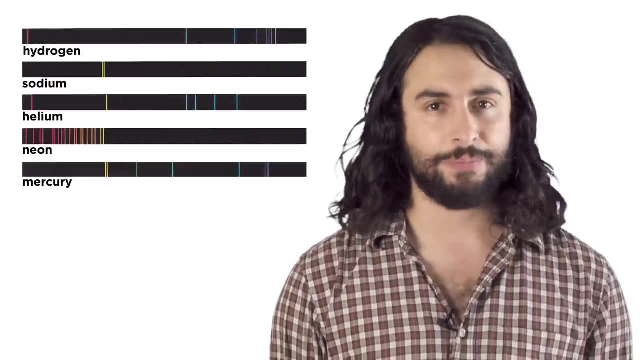 atom has positively charged protons and negatively charged electrons. why are atoms stable? why don't the electrons just collide with the nucleus? and what were these emission spectra that we can see? what is it about different elements that makes them emit light of different colors? Bohr answered these questions. 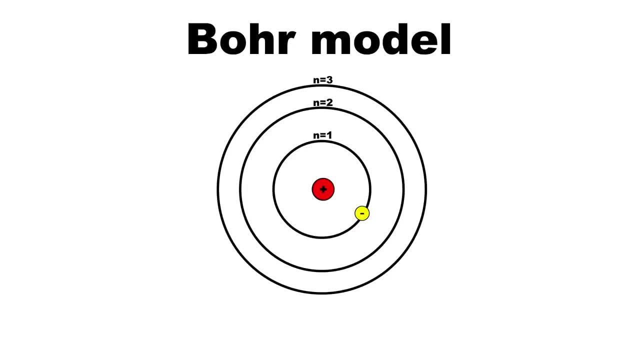 with his model of the hydrogen atom, he extended the idea of energy quantization and said that the potential energy of the electron in a hydrogen atom is also quantized. this means that an electron can't have any imaginable energy, but can only inhabit certain energy levels. 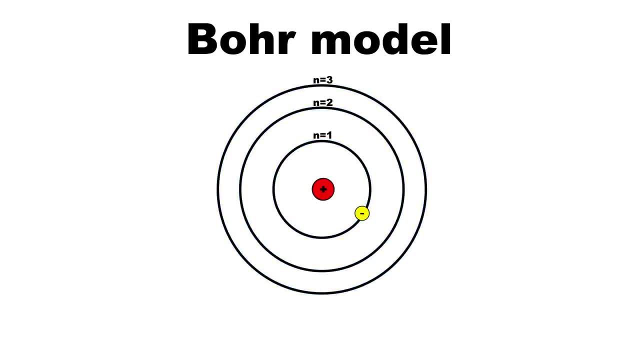 that are at fixed distances from the nucleus. each type of atom has its energy levels at different values due to its unique number of protons in the nucleus, and an electron will transition from one energy level to another when a photon of a very specific energy is either absorbed or emitted by the electron, the 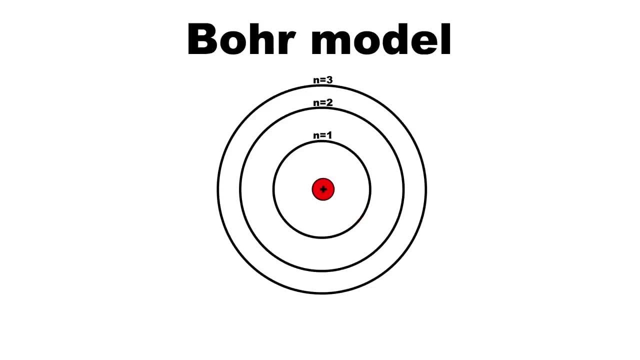 energy of the photon will correspond to the difference between the two energy levels. so if the electron in a hydrogen atom goes from the n equals three to the n equals two energy level, a photon will be emitted that is equivalent to that specific energy gap. another transition has a different. 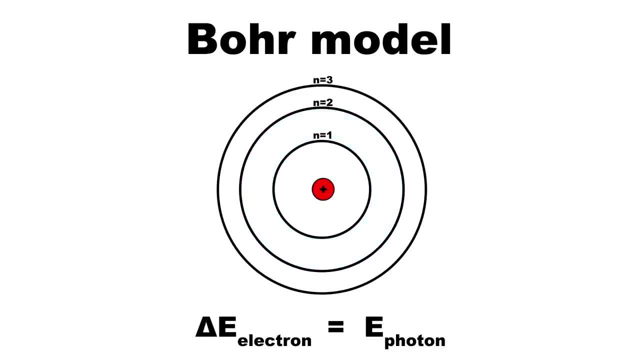 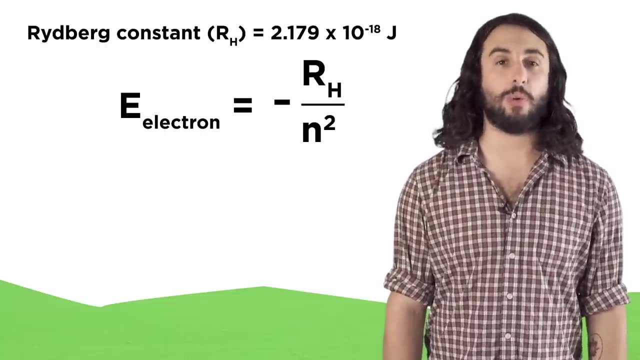 energy gap associated with it and therefore generates a photon of that particular energy. and to go from lower to higher energy levels, an electron must absorb a photon of that particular energy. for a hydrogen atom, the energy levels depend on the Rydberg constant and are given by the following equation: 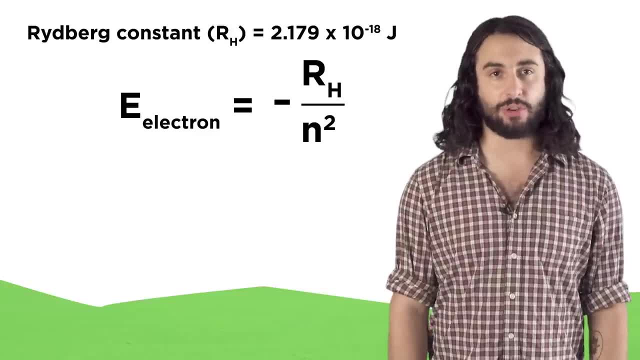 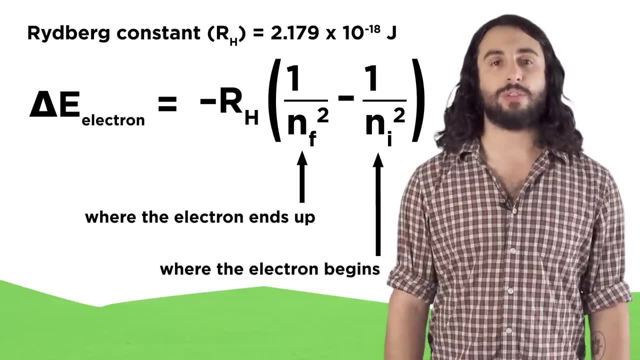 but we typically just measure the change in energy of an electron during a transition. so we can modify this equation to include the change in the energy level. n final is where the electron ends and n- initial is where it begins. using this equation, we can predict the wavelength of photon. 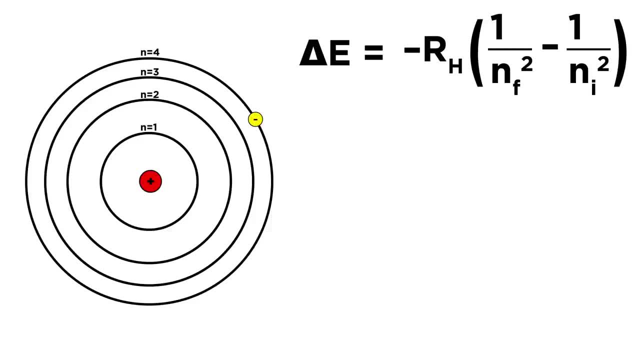 associated with any possible transition for the hydrogen atom. take this transition, for example, from four to two. plug in where the electron starts and where it ends and we get the change in energy of the electron, which equals the energy of the photon. from energy we can get frequency.